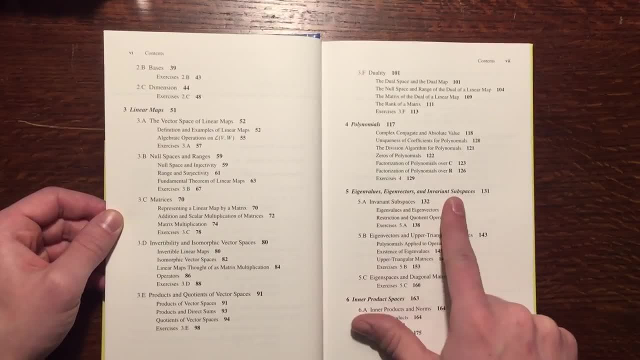 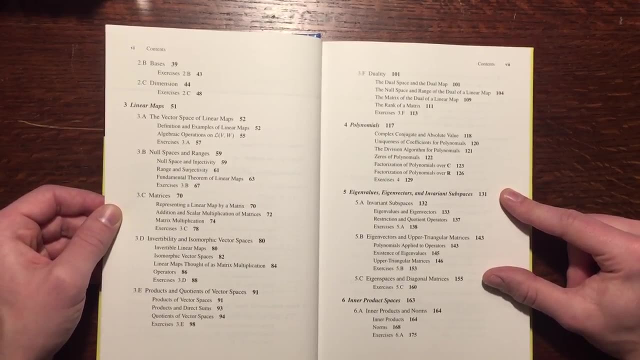 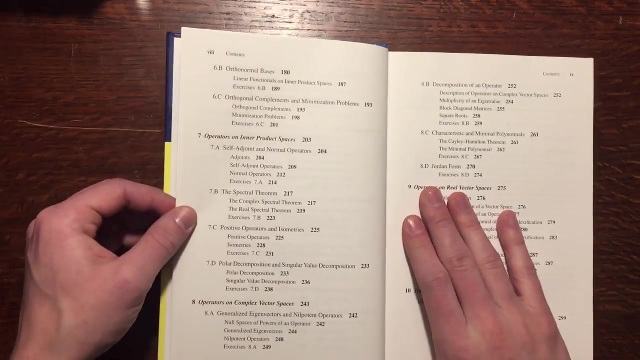 A little section on polynomials, Eigenvalues, eigenvectors, Huge right Eigenvalues and eigenvectors have so many applications in many areas of mathematics- Interproduct spaces, So that talks about some stuff you might be familiar with, like dot products is one example of those things. 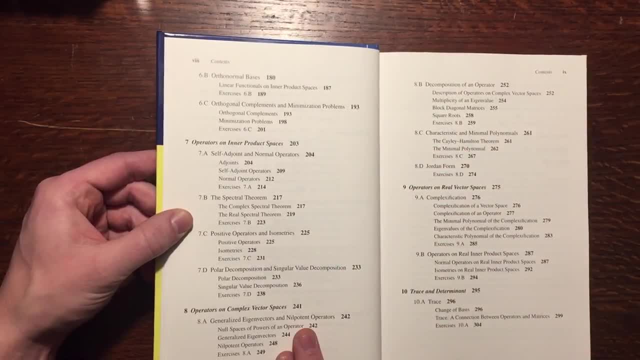 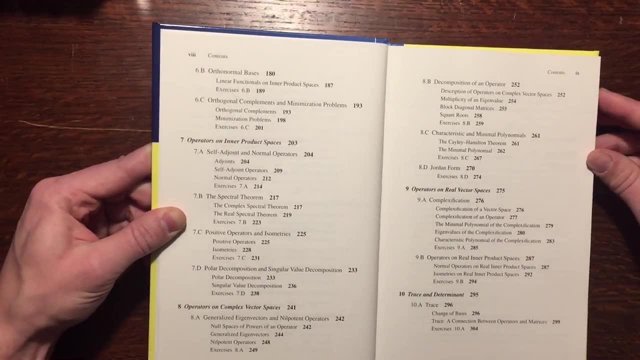 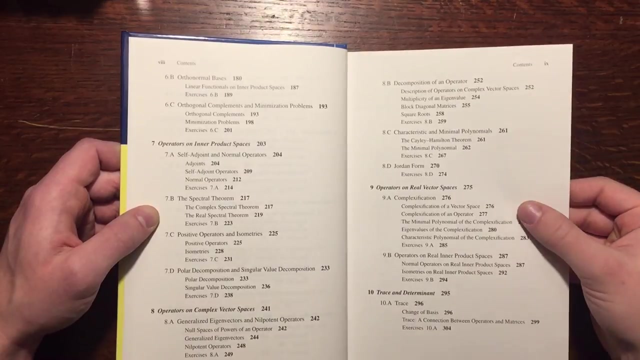 Operators on Interproduct spaces, operators on complex vector spaces and operators on real vector spaces. Personally I don't know too much about that stuff yet, but hopefully I will soon- And chapter tens on trace and determinants. So these are two things that you might have seen before if you were taking a matrices class. 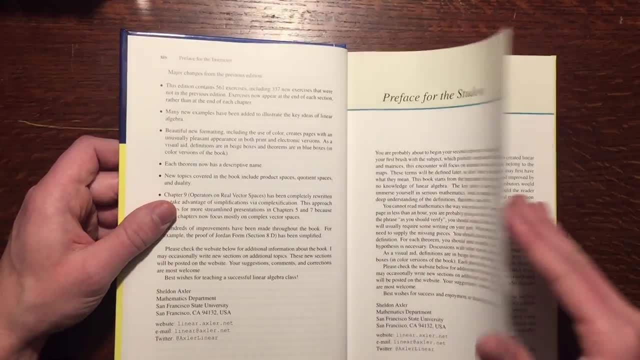 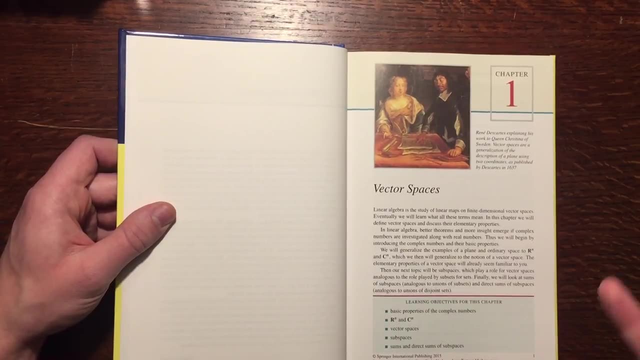 As far as how this book is laid out, it is very for the student because it's a good way to keep track of things, But I don't think it's just for the student here. it's very readable- most advanced math textbooks. you can't really well, maybe you can, maybe you. 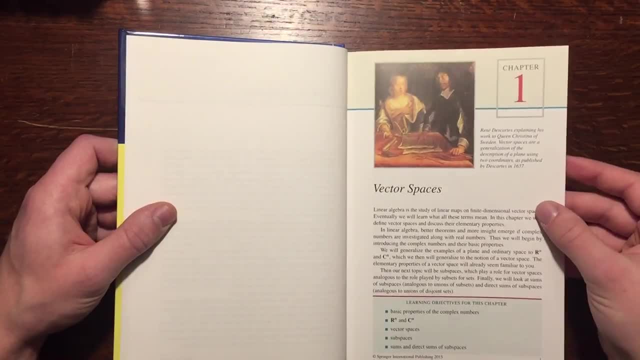 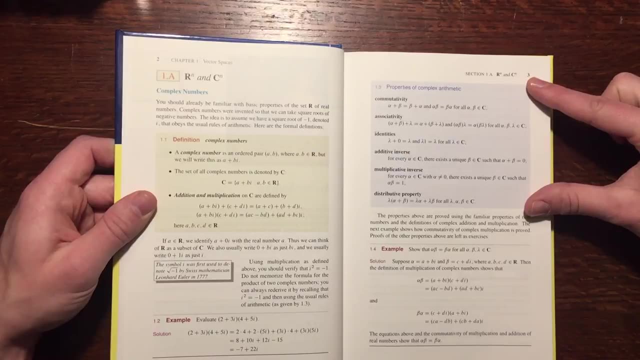 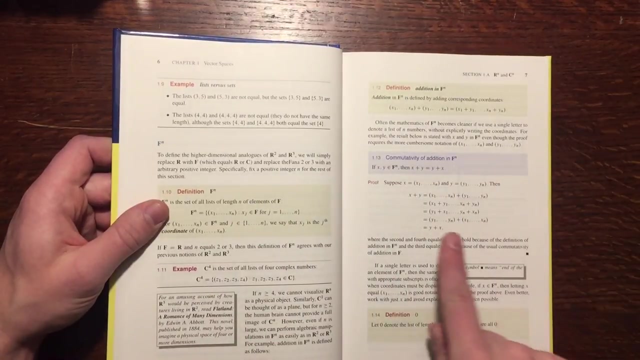 can't teach yourself or maybe it's really hard to read. you gotta like slog through it. but this one is really intuitive. it does what I love the textbooks do. they highlight all the important things. they put examples after it, then, and they have hopefully have an example here. there's like 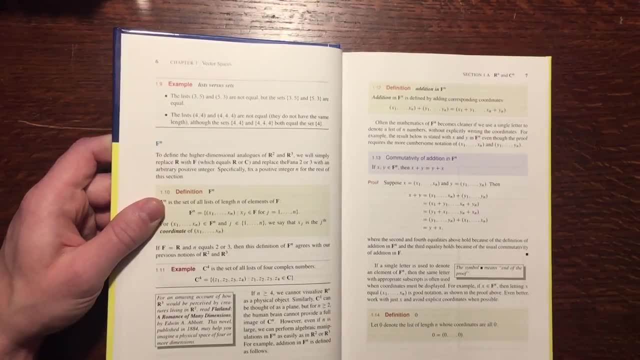 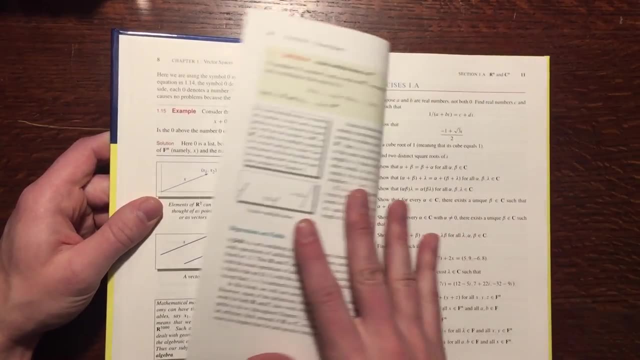 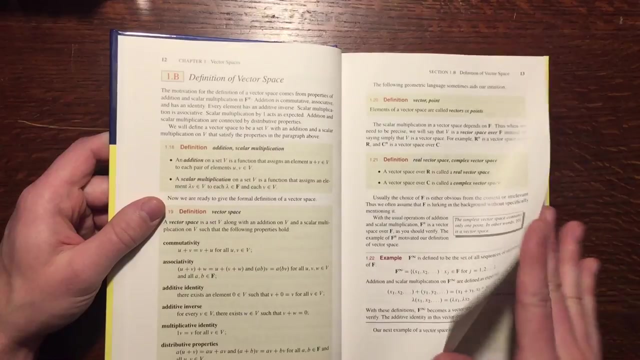 proof worked out right for you. it's really nice. you can maybe get a cup of coffee and sit down for an afternoon and teach yourself this stuff- no professor required, which is really nice. and of course, at the end of each section there are many examples- maybe 20 or 30 per section- which 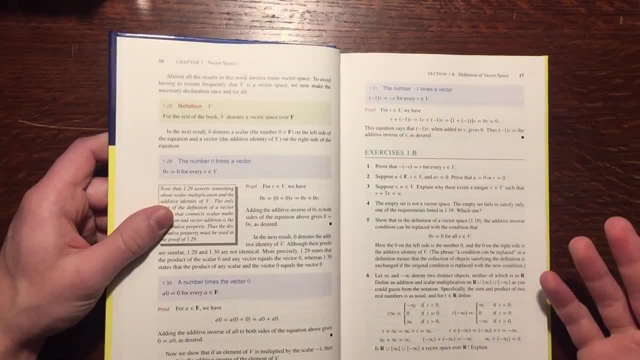 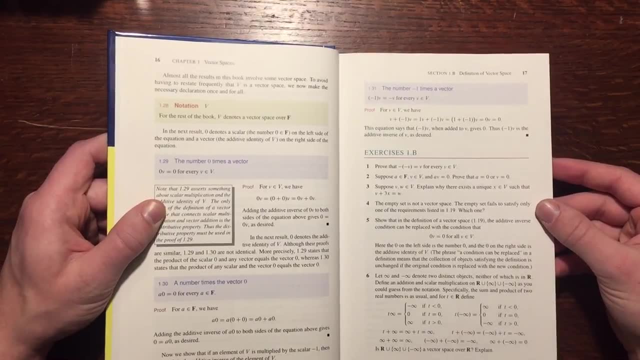 is really nice and they're totally doable. this is an advanced math textbook, so I don't believe the answers are in the back, or even available anywhere, maybe. but at this point in the in your mathematical career, if you have this book, um, you should, you should pretty much be. 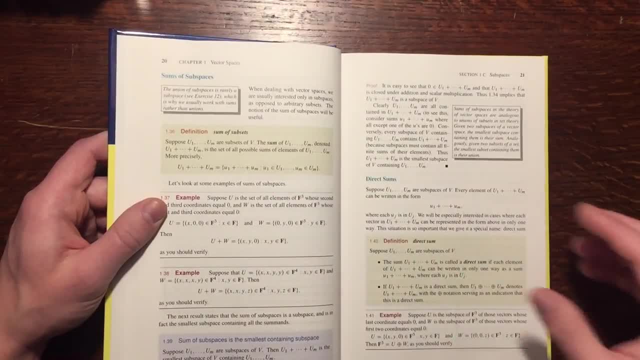 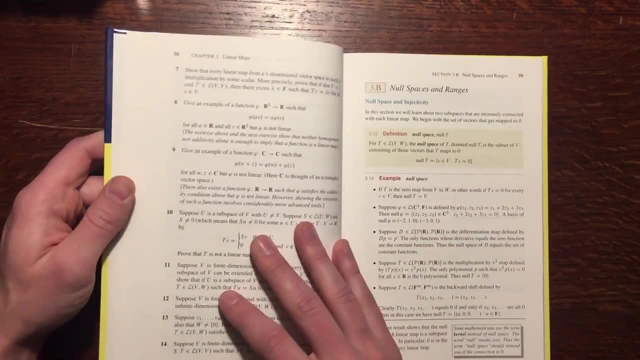 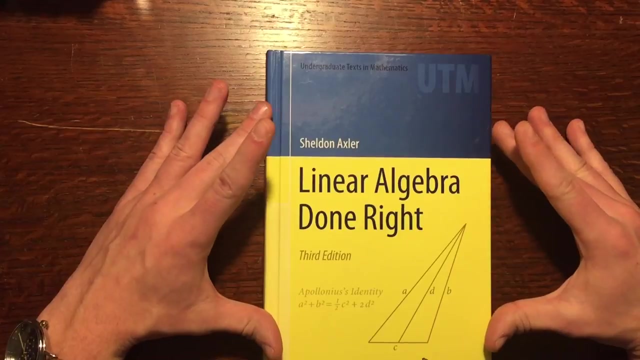 able to know whether you're correct or not. maybe that's not very comforting to hear it's- it's. I gotta tell you it's a great book. if I were to recommend a linear algebra book to someone who is taking a more advanced linear algebra class, this would be the one. I think this 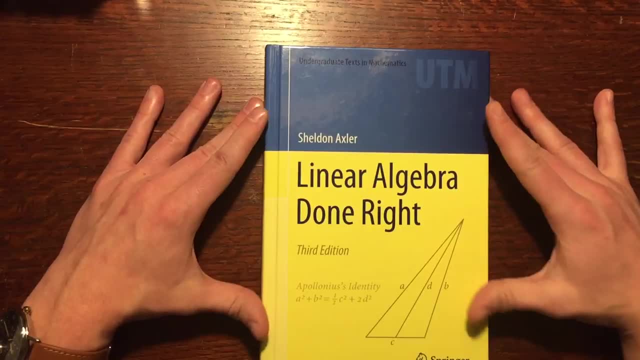 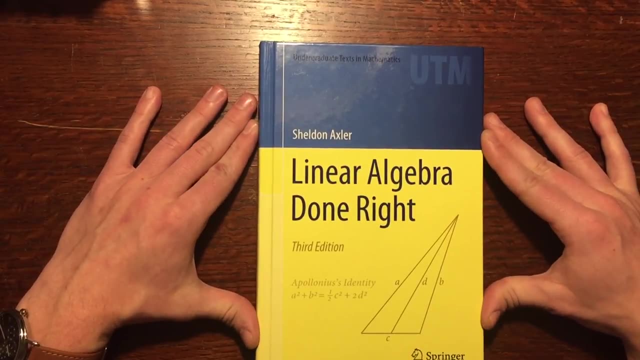 book is true to its name: linear algebra, done right. this is, in my opinion, how the course should be taught and introduced. so if you're interested in looking at this one, I'll throw a link in the description. you can check it out. I think I got this for around 40 or 50. 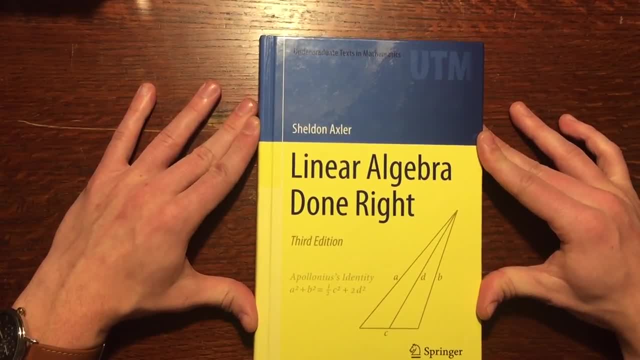 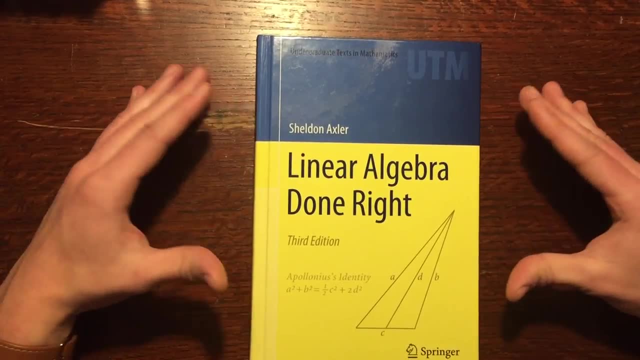 dollars new. I'm sure you can get it cheaper than that used or rent, depending on what you want to do, if you poke around a little bit. anyway, I hope you enjoyed this video. hope you found it informative. maybe you got an idea of a book you might want to get, should you be. 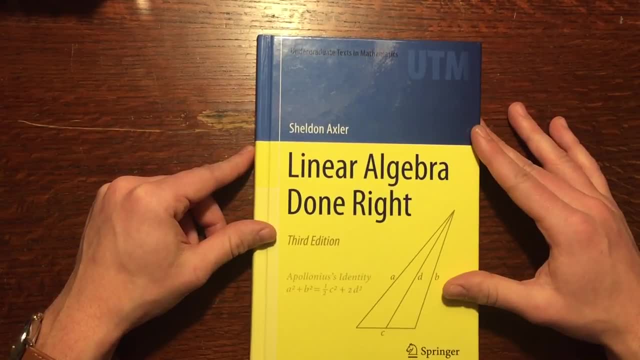 taking an advanced linear algebra class. and thanks for watching again. have a great day. bye you. 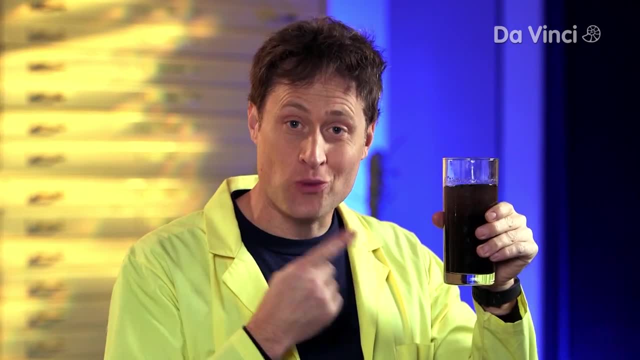 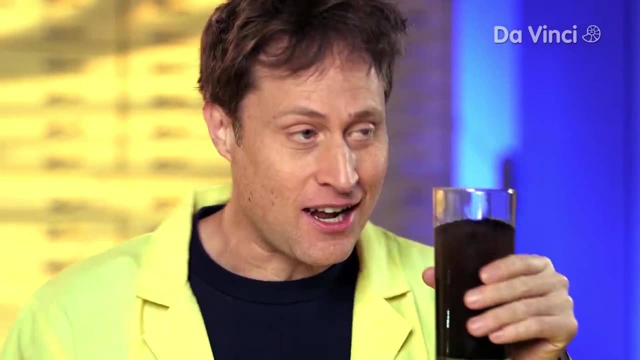 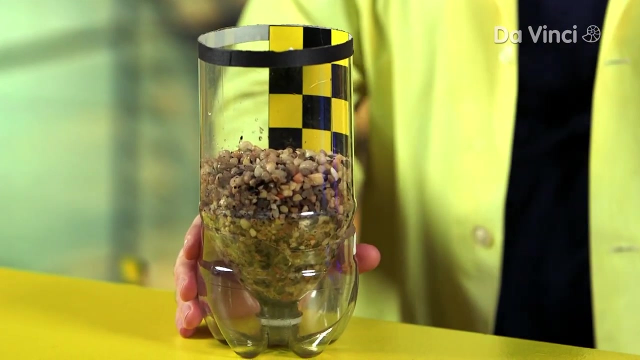 Ew, this water is gross. but I'm going to drink this water. Why? Well, because of science. No, but I'm not going to drink the water like this. First, I'm going to use the power of science to help me clean it. How? By using gravel. Gravel, yes, gravel, So say I've. 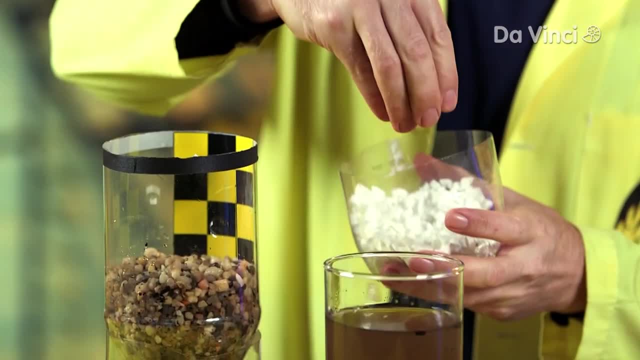 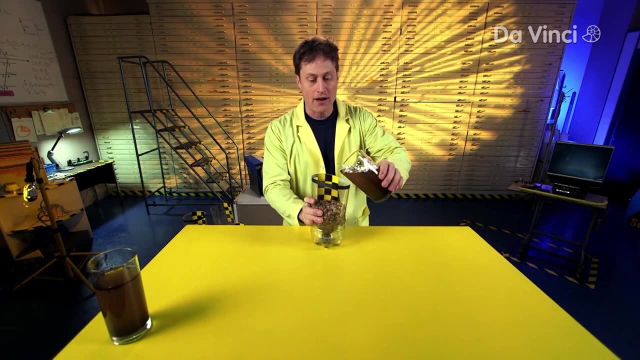 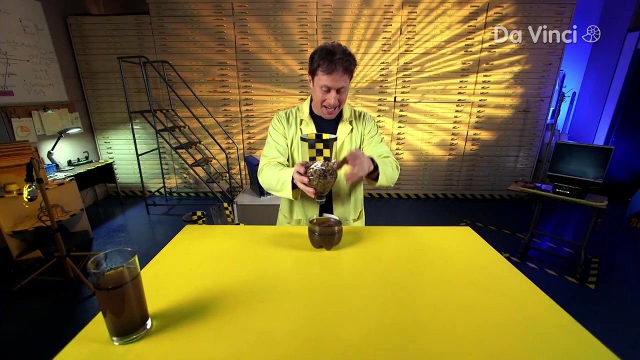 got some dirty water and there are particles floating in that water, Large particles. your rocks, your wood, these styrofoam bits will act as the large particles. You pour it into the gravel and the large particles get filtered out. See, Nothing but clean, clean water. 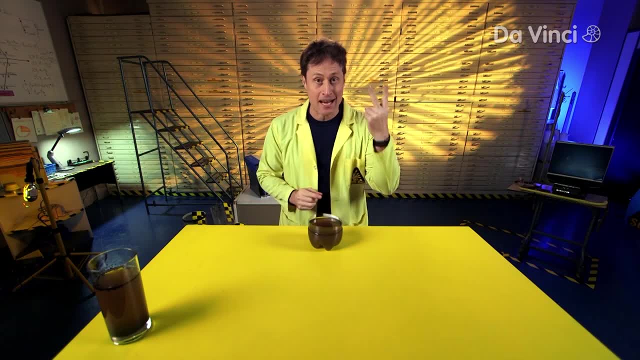 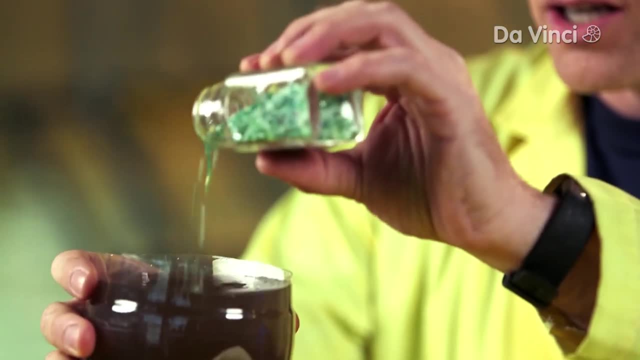 Yeah, I know what you're thinking, Phil. that's not really clean yet. That's because we haven't done step two. Sand, Sand, Yes, sand. Let's say that these plastic beads are small particles. That filters out the tinier stuff. 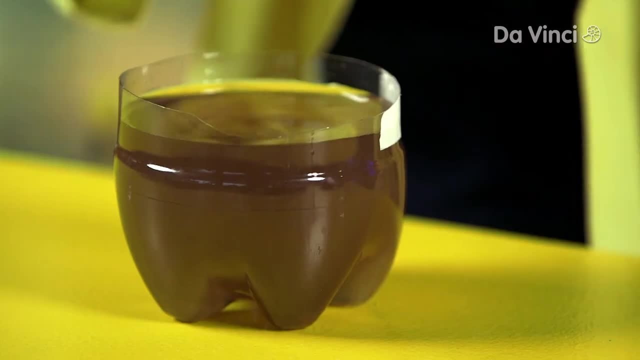 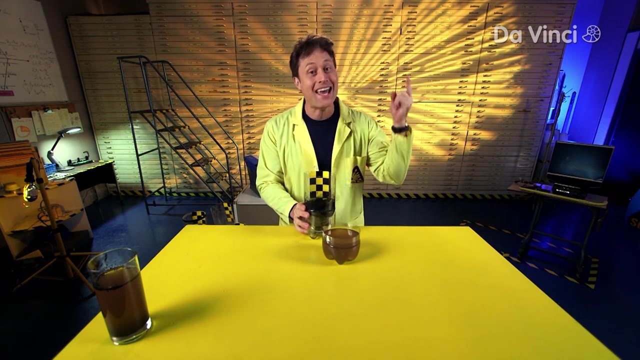 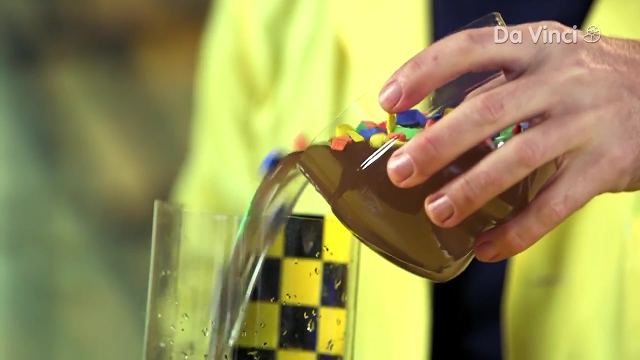 There, Huh, Clean, right? No, it's not very clean. So we filter the water in the next step with charcoal. What Charcoal? Yes, charcoal. Charcoal works just like gravel and sand, except on a microscopic scale. Say, these bits are tiny particles, you can't even see The 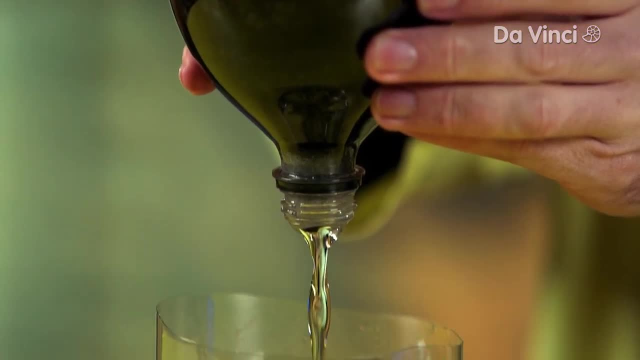 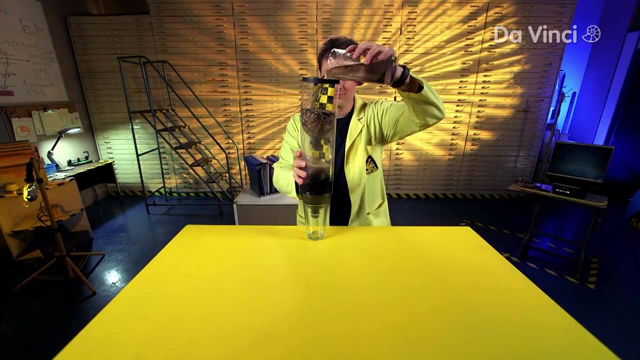 charcoal catches these, like the sand, and gravel caught the larger particles. This is called a gravel, sand and charcoal filter. The gravel filters out the tinier stuff, Charcoal catches the big particles, the sand the smaller ones and the charcoal the 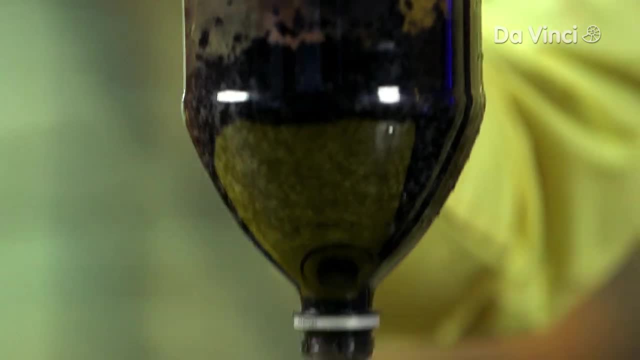 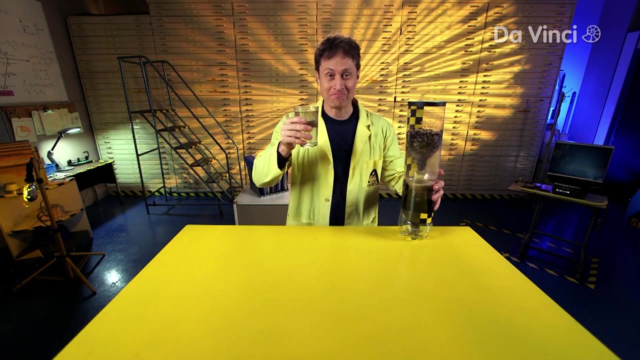 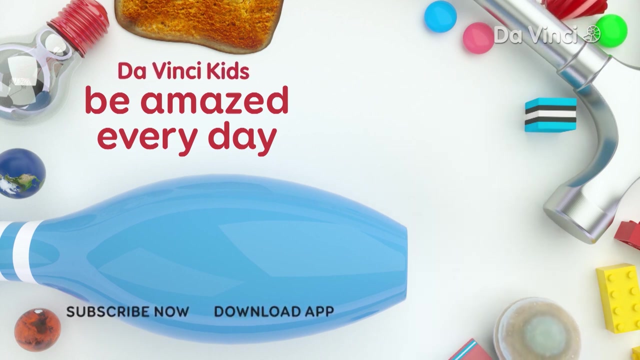 microscopic ones. These kinds of filters are used all over the world to clean drinking water. Ah, Delicious Science. I've never thought of that. So the concrete is good. Yeah, I'm a little bit of a project student myself. I love being a computer scientist. That's cool. There are a couple of options, though. There's one way of doing this. Let's try this. Yeah, Let's try it. Okay, Okay, Yeah.